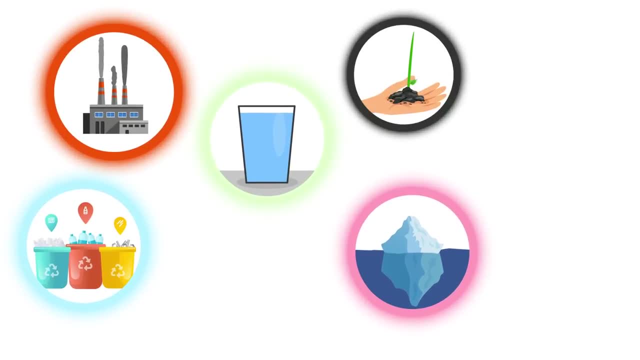 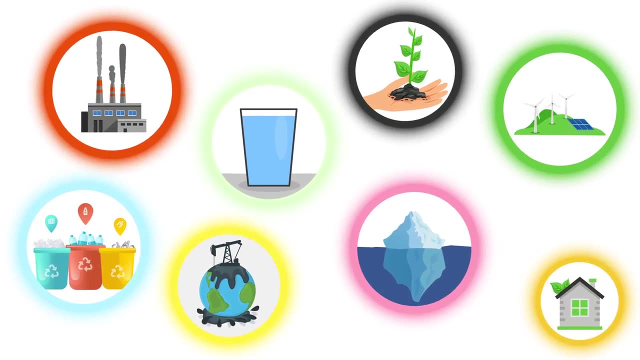 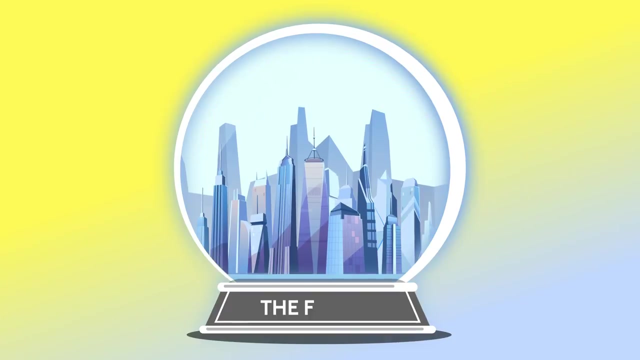 From water, waste removal, pollution control, food building regulations, public health, clean energy. the list is endless, And it's down to the environmental engineers to ensure our needs are met, all whilst protecting our planet for future generations. This means looking into the future. If the population of London doubles, 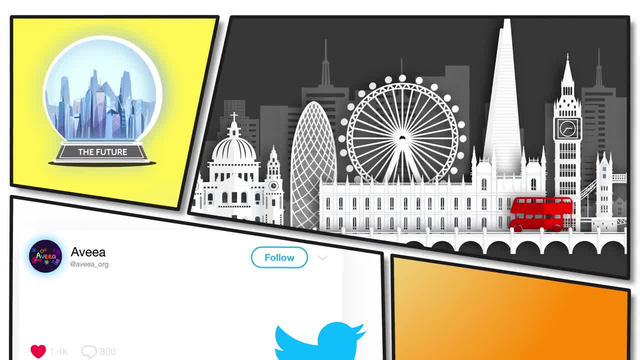 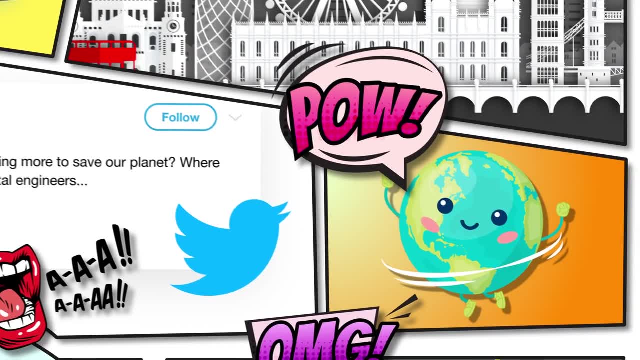 will everyone still have access to all these resources? That's not to mention. every day, someone is talking about rising CO2 levels, and rightfully so. We only have one planet and the way things are going, we definitely need to make some changes If we continue producing energy with our old fossil. 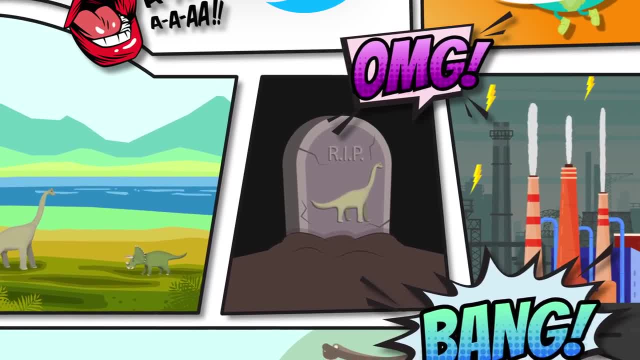 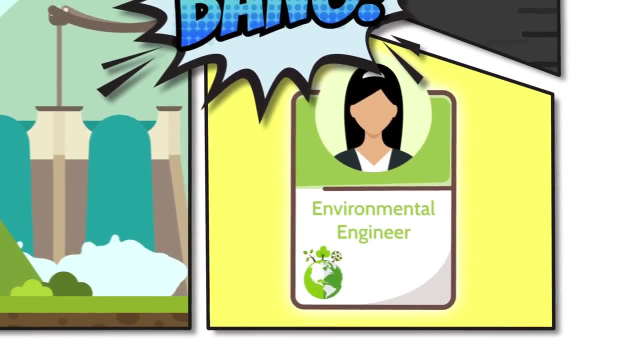 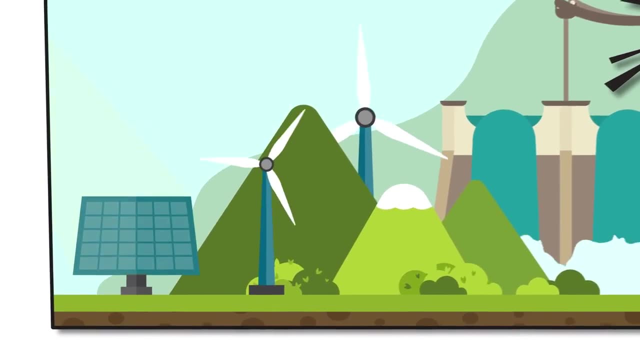 fuels, in other words, burning dead dinosaurs to produce electricity. what's going to happen to our planet? So you're probably thinking: ah yes, environmental engineers look at renewable energy solutions like wind, solar and hydroelectric power. But it's not all about that. Allow me to explain. Let's look at solar power. 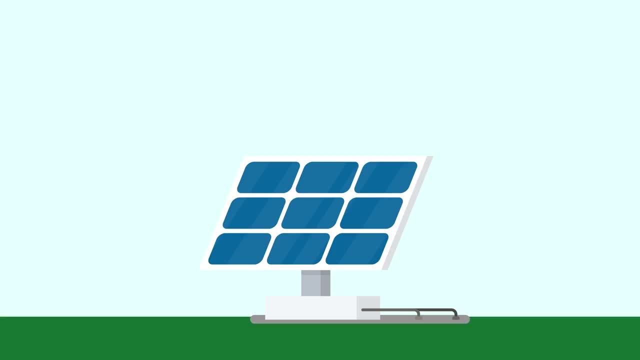 it's something we all know quite well. The main part of a solar panel is silicon. This is what allows the panels to convert the sun's energy into electricity. Now, to do this, we need to start with a rock-like substance like quartz. 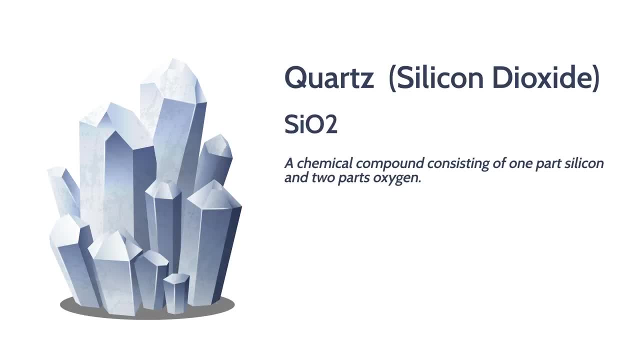 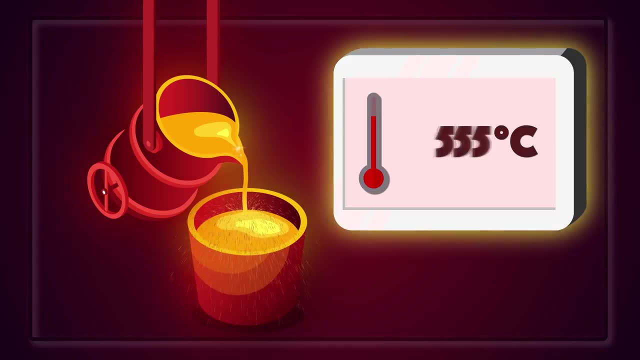 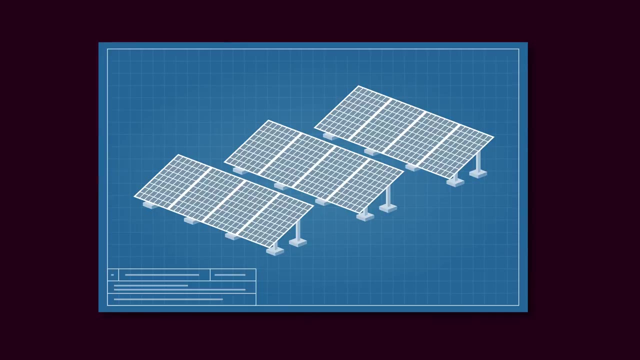 also known as silicon dioxide. This needs to be purified to create pure silicon and CO2, which is done by heating it up to nearly 2000 degrees. Can you imagine the amount of energy needed to melt rock? Yes, rock, And it is this silicon that is put into our solar panels with. 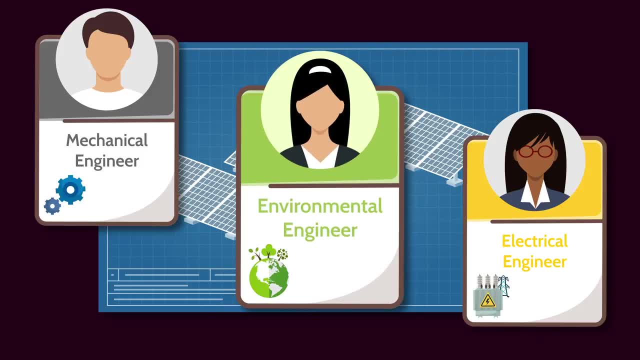 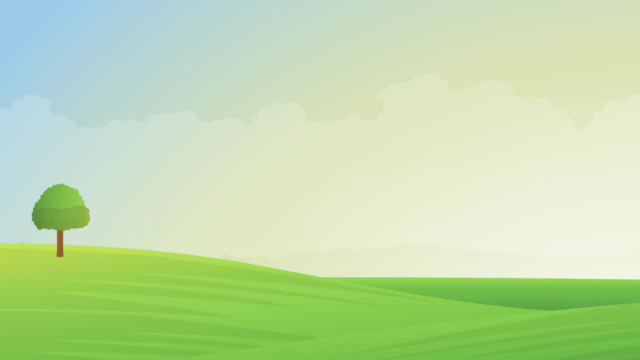 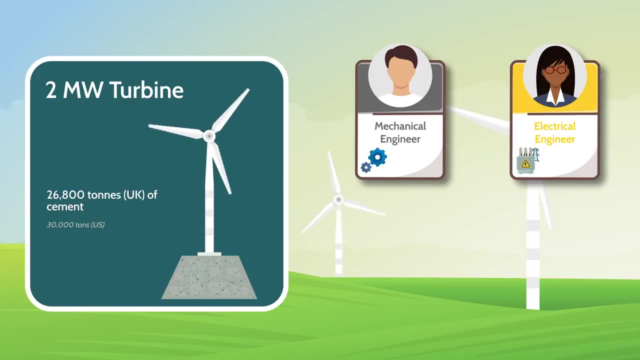 the help of mechanical and electrical engineers. So hang on a second. where do environmental engineers fit into this? Well, hold on to that thought. Now for wind turbines. aside from the main turbine itself, which is designed again by mechanical and electrical engineers, there's also the foundations to think about, which is made from concrete and 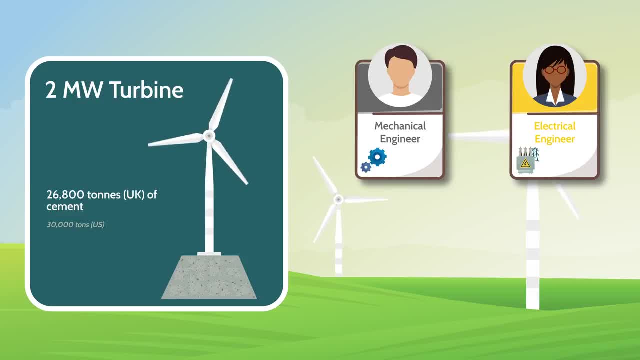 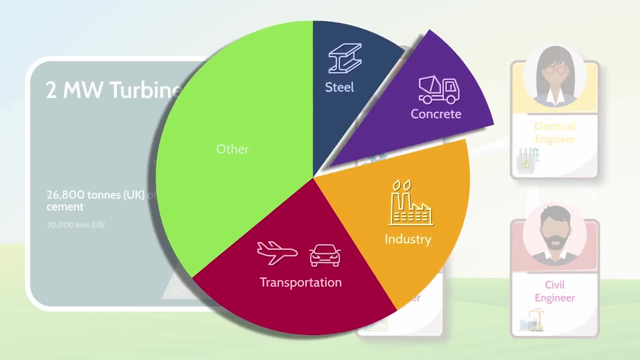 reinforcement to hold the structure in place, which, of course, is designed by civil and structural engineers. But here's a fact you might not know: The production of cement, the main material to make concrete, is responsible for around 7% of annual carbon emissions. Oh, and not to forget, 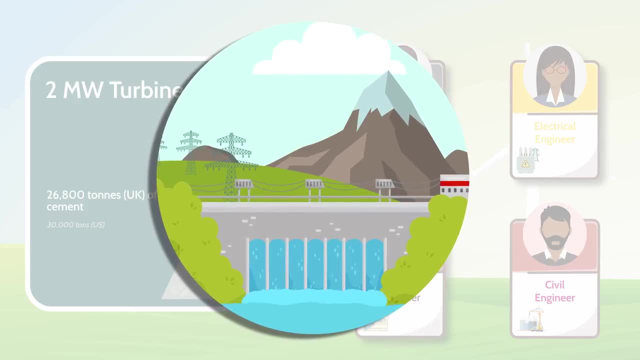 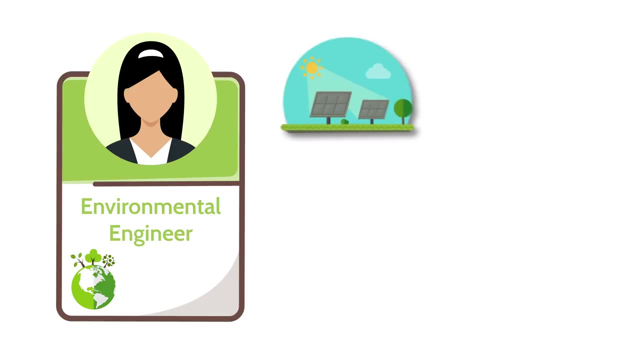 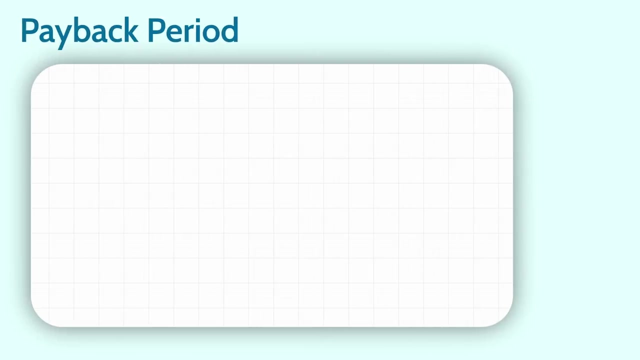 hydroelectric dams, the amount of concrete needed for them. Have you seen the size of those things? So enough with all these different engineers. what about environmental? Well, you can probably notice a bit of a trend with creating these renewable energy sources and the energy they require, And this is where something called a payback period. 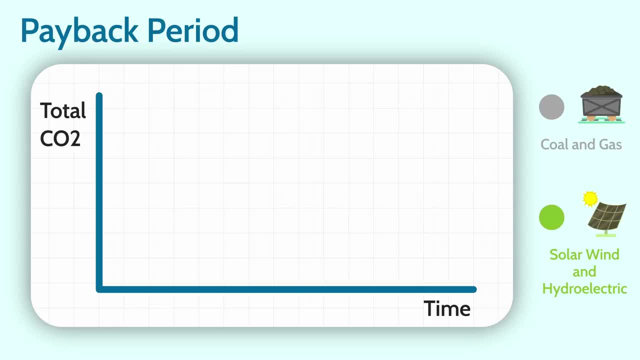 comes in. Think about it this way: coal and gas power stations are churning out emissions every day, And although solar, wind and hydro produce enormous amounts, before operation, once operating nearly nothing. But imagine if that solar panel only lasted five years. 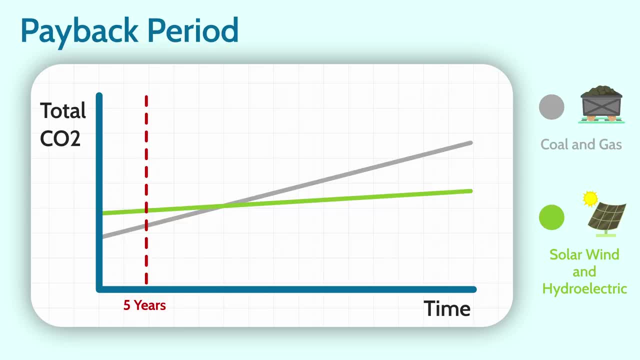 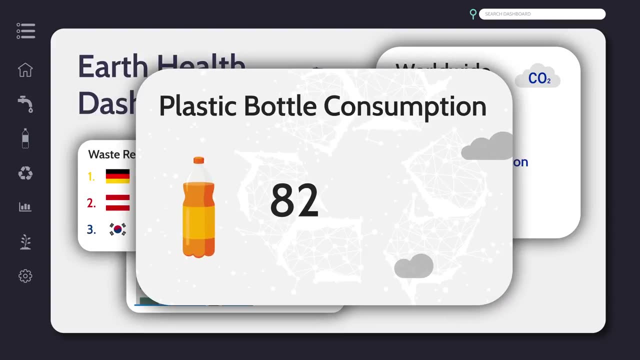 The negative implications of this could be worse than a coal powered station, And this is how environmental engineers look at the planet: holistically, Like plastic bottles. It's not really about the one bottle that produces 82.8 grams of CO2 when manufactured. 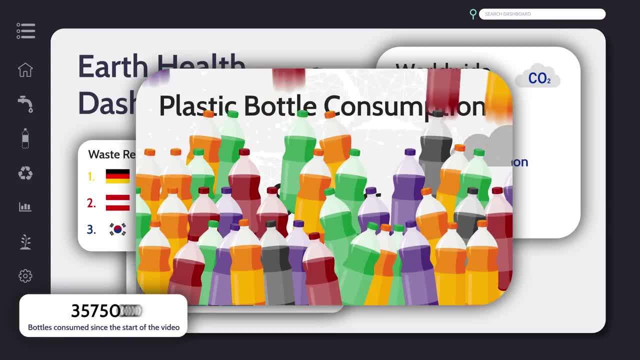 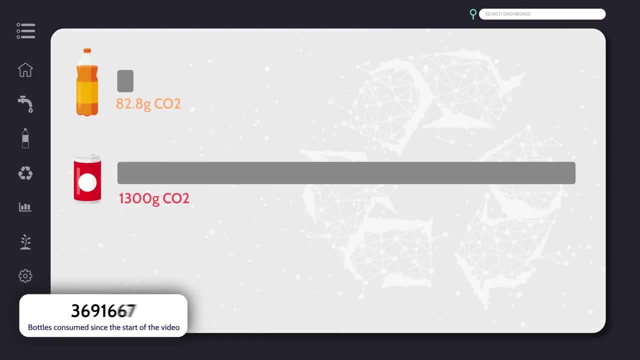 It's the fact that us humans buy over a million of them every single minute. To make that worse, aluminium cans. That's close to 1,300 grams of CO2 per can, The same as a car driving around for five miles. 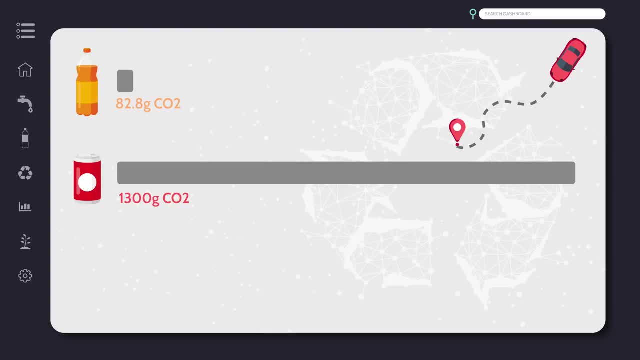 That's just mind-blowing to think So for environmental engineers, they need to look at making the most out of these materials. For example, if you were to recycle this aluminium can, this could save 95% of the energy needed to make this metal again. 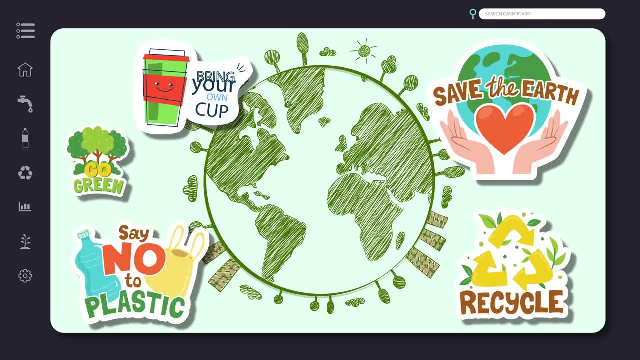 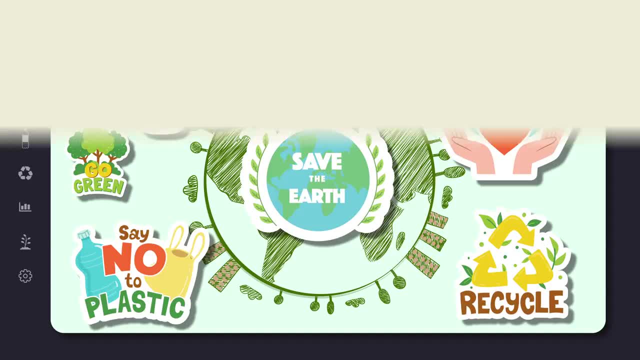 You can see why environmental engineers are so keen on improving recycling techniques. They're always looking into what's causing problems to our Earth and where our efforts should be focused. Sometimes the problems are huge, like the BP oil spill Engineers here. look at all different biological species. 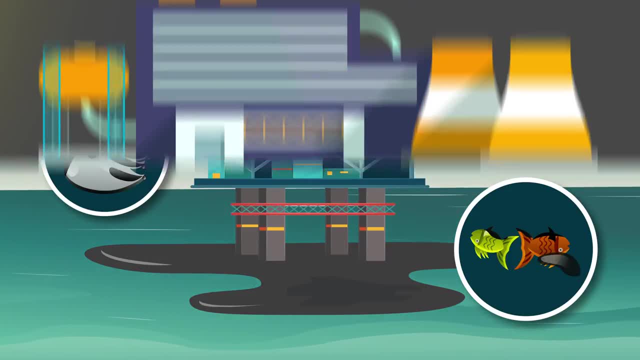 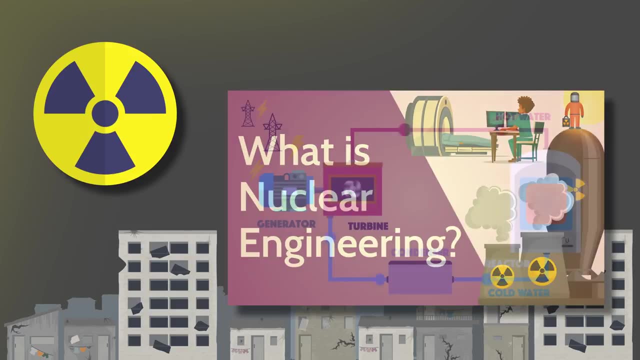 and the chemistry of the ocean and how it's been impacted, Or Chernobyl, and assessing whether it's safe to actually live in such an ecologically destroyed area. If you want to know more about this, we've done a great video on nuclear engineering. 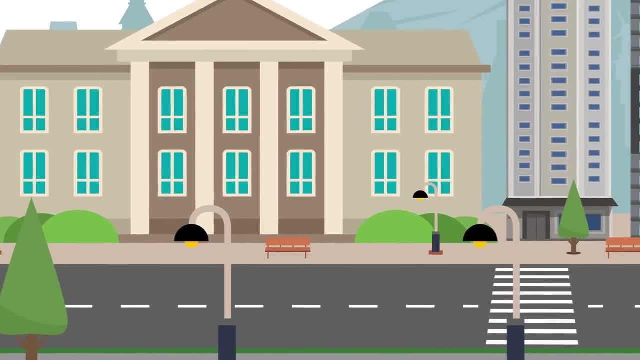 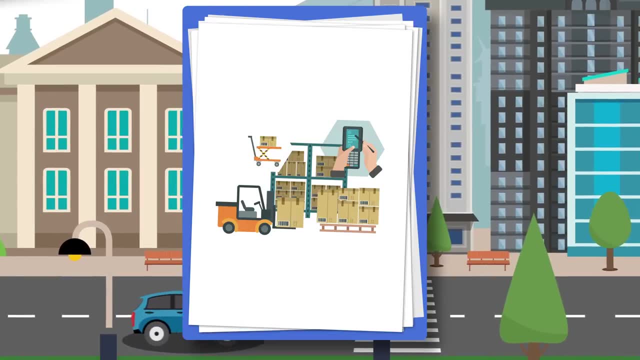 And it really isn't an Avia video- without mentioning how they helped the government. Think BREEAM, a body that assesses how sustainable a building is From how it was constructed, how it operates. what demolition would look like. can some of these materials be reused? 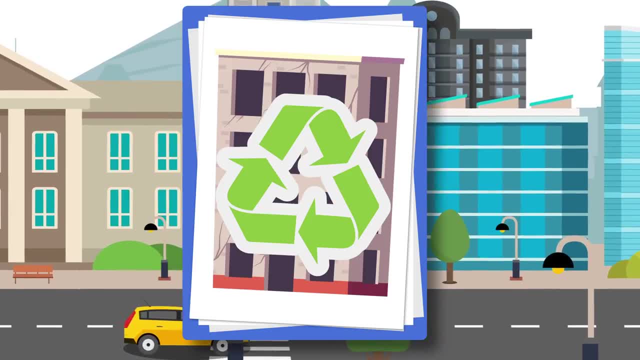 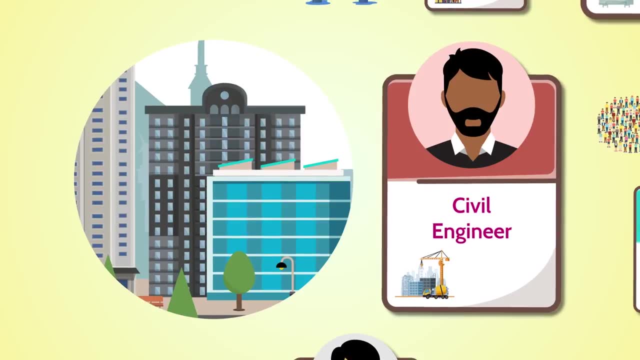 when we no longer want this building in place. I mean, things do go out of fashion, even buildings. So working very closely with civil engineers to get sustainability designed from the core is critical, And really that's what it boils down to.